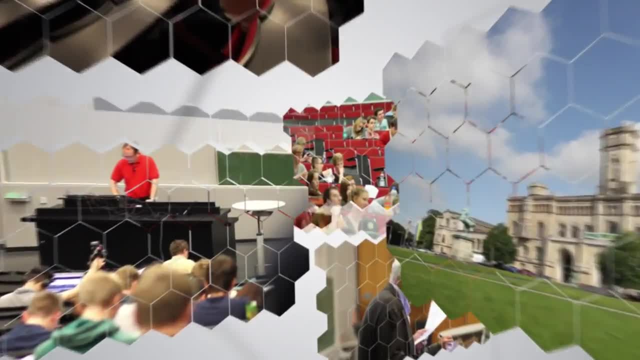 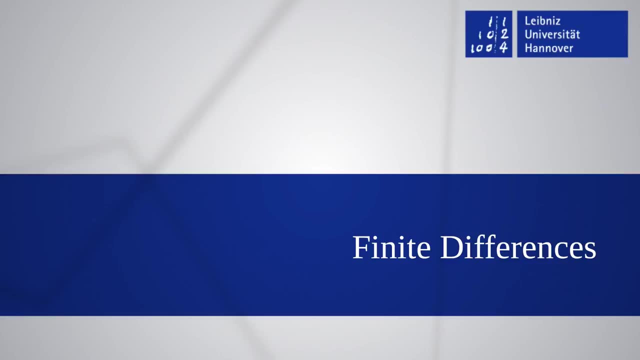 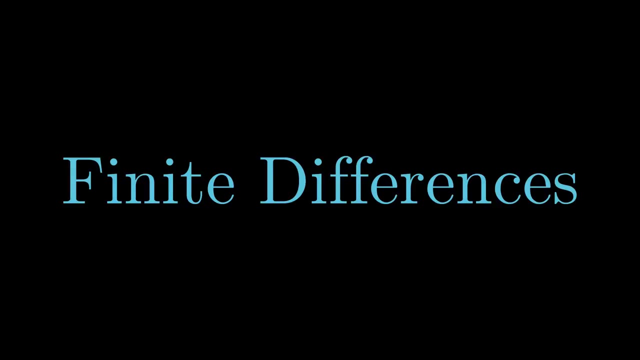 For many centuries, scientists have been trying to solve differential equations. Often, it is difficult to solve these problems by hand, or it might even be impossible. Therefore, we will now take a closer look at a very simple method to approximate partial differential equations- PDEs, which is still used in 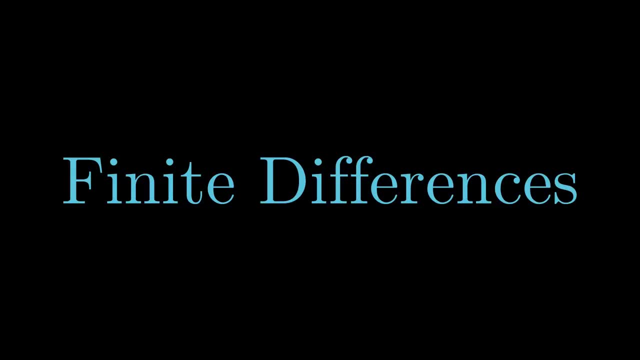 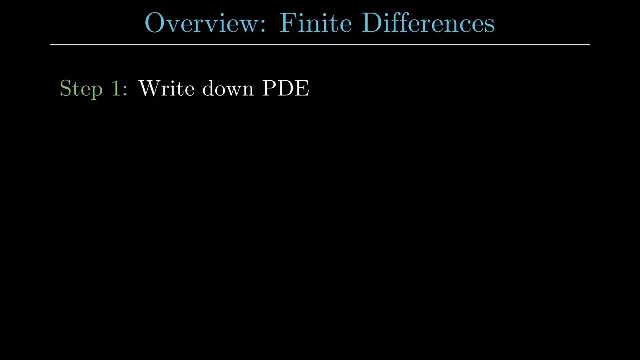 the industry. Let me give a quick tour of finite differences. Overview finite differences. The finite difference method consists of the following steps. Step 1: write down the PDE: What is our problem description? Step 2: decompose the domain. We make our problem finite dimensional. Step 3: approximate derivatives- Insert. 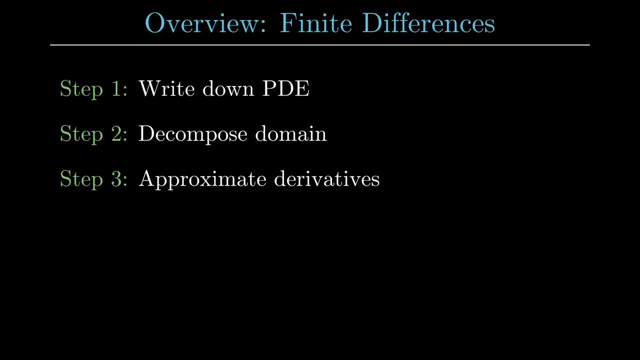 finite difference, approximations for derivatives into the PDE. Step 4: assemble linear system with finite difference. stencil. We write the PDE that has been approximated with finite differences and discretized on a grid as a linear equation system. Step 5: solve the linear system. Step 6: visualize and. 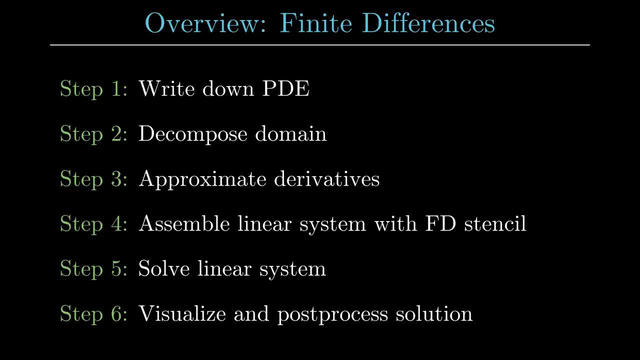 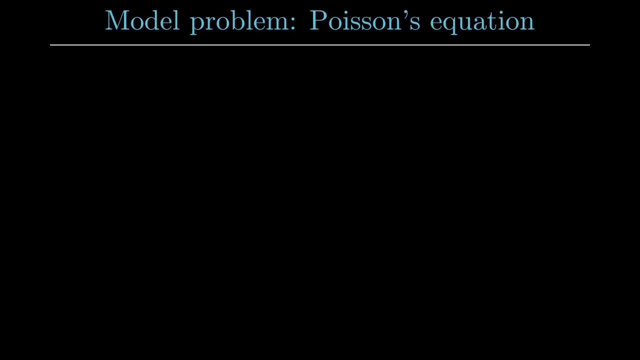 post-process solution. We have to answer the following questions: Firstly, is our solution plausible? Secondly, how good is our approximate solution? Quantitative error estimation. And finally, is our solution possible? How quickly does our approximation converge to the analytic solution? Computational convergence Model problem- Poisson's equation. Let us now analyze our 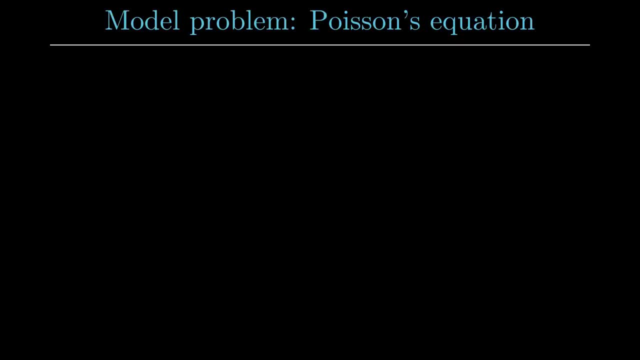 model problem, Poisson's equation. It reads: minus Laplace, u equals f in the domain Omega and u equals 0 on the boundary of the domain. Now we have to specify how the Laplace operator does the approximation. The Laplace operator will define theey sum of derivatives with respect to x due to the 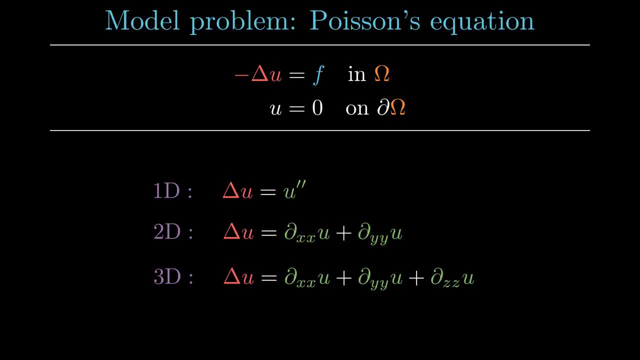 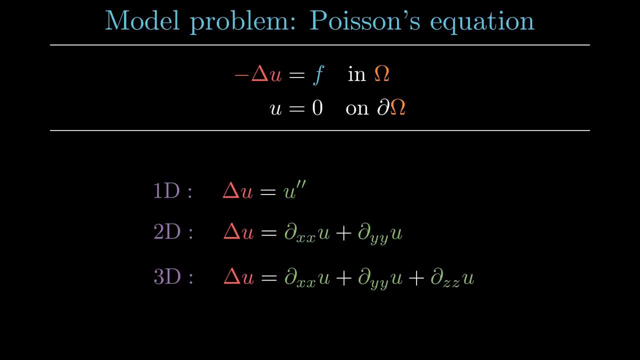 of h. All this we'll write in the Write gives us. now we need to find the respect to y In 3D. the Laplacian contains also the second derivative with respect to z In the following we will restrict our analysis to the two-dimensional case and can. 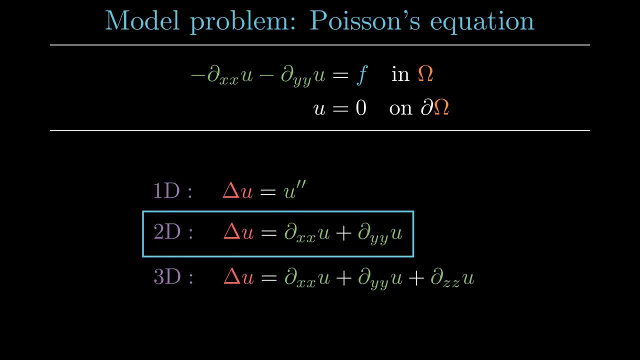 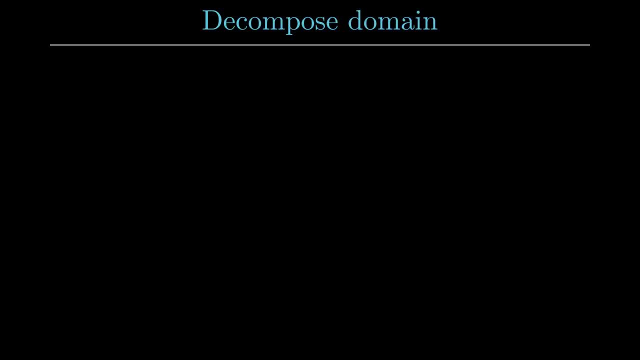 thus insert the definition of the Laplace operator into the Poisson problem. Decompose domain. Until now, we haven't specified on which domain we are solving the Poisson problem. In this video we will work with the L-shape, which is a square from minus 1 to 1, from which the part inside the first quadrant, its upper, 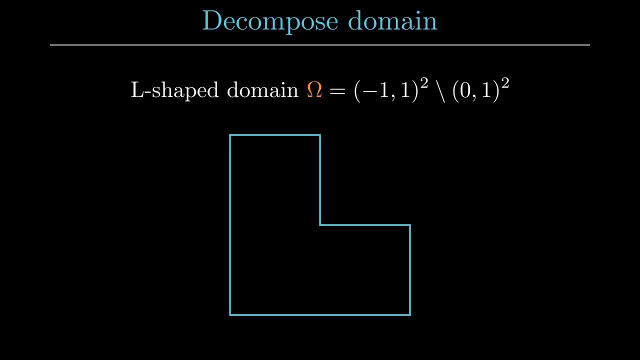 right corner has been removed. To reduce Poisson's equation to a finite-dimensional problem, we now need to only solve the PDE in a finite set of points from the L-shape. This can be done by dividing the domain with a grid. 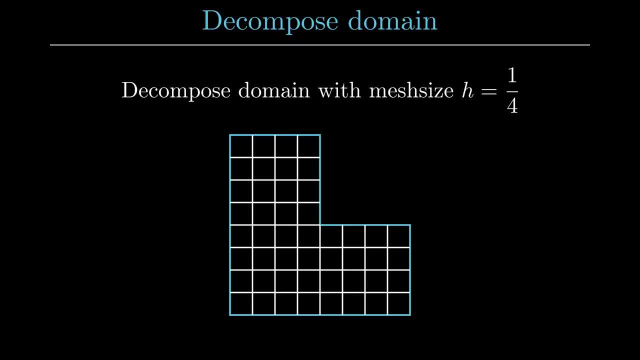 Here the mesh size- h equals one quarter- is the distance between two parallel grid lines that are directly next to each other. At each point where two grid lines intersect, a point ui is placed and the equation minus Laplace u equals f, needs to be fulfilled. 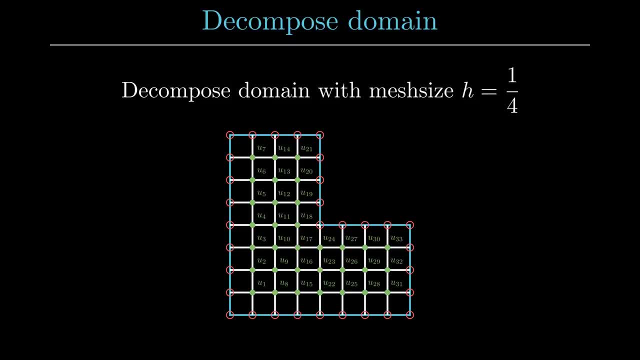 there. Furthermore, at the points on the boundary, the red circles, the solution should be zero Decompose domain. Until now, we haven't specified on which domain we are solving the Poisson problem To reduce Poisson's equation to a finite-dimensional. 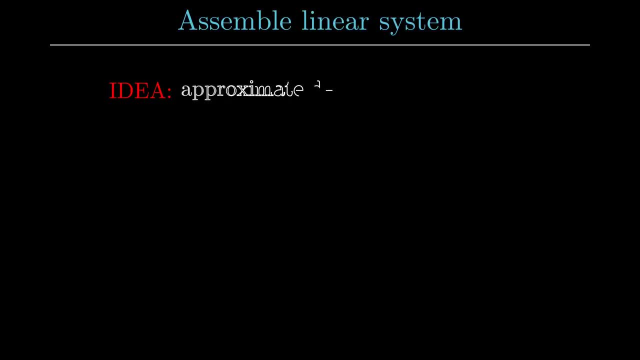 problem. we need to only solve the Poisson problem. To reduce Poisson's equation to a finite-dimensional problem we need to use the Poisson's theorem Assemble linear system. The core idea of the finite-difference method is to approximate derivatives in the PDE by difference quotients. The formal definition: 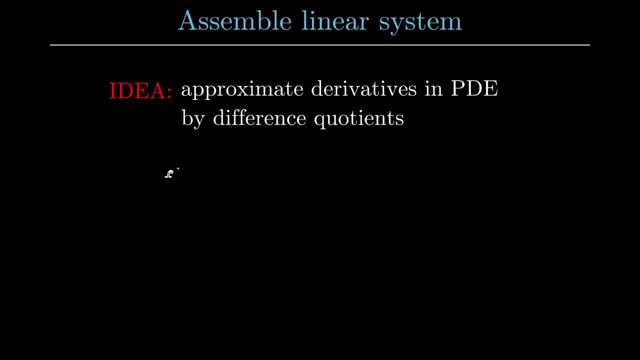 of the derivative is f' is the limit of f minus f over h, as h goes to zero. Please note that for small values of h, this quotient is a good approximate of the derivative. However, in the Poisson problem we only have second derivatives. 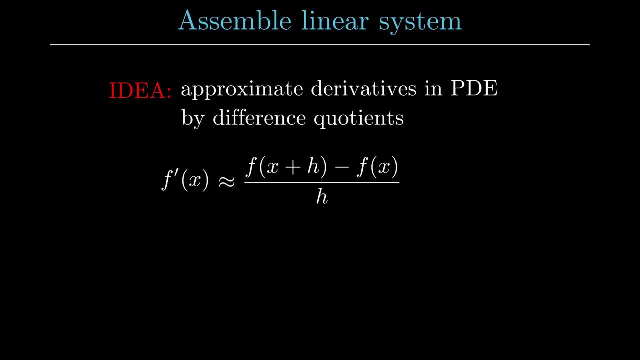 For the second derivative we get by Taylor expansion that f double prime of x is approximately f of x plus h minus 2, f of x plus f of x minus h, all over h squared, which holds true for small values of h. This formula is called the. 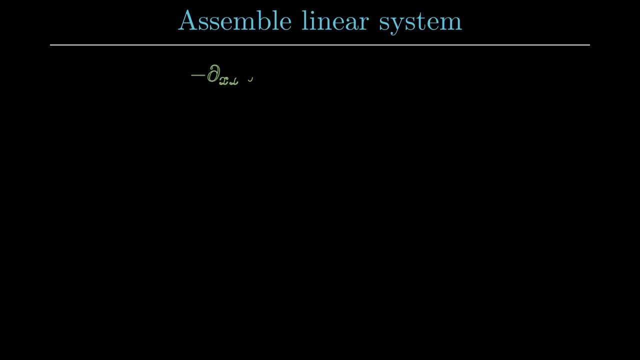 central difference quotient. Now let us go back to Poisson's equation. If the equation should be fulfilled on the entire domain, it should also be fulfilled in our grid, points u1 up to u33.. Here we use the notation ui for the value of u. 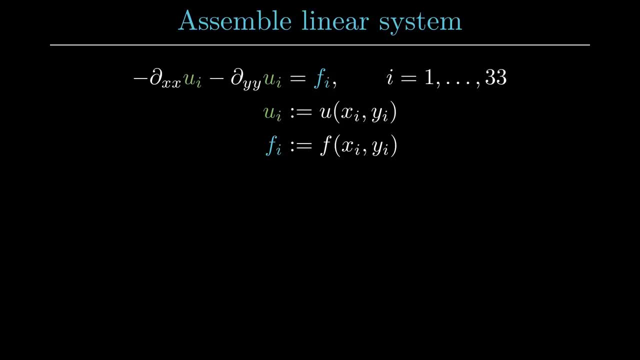 at the i-th point and fi for the value of u at the i-th point. We can then approximate the second derivatives of u with respect to x and y by the central difference quotients and insert these formulas into the PDE. This can be simplified to one over h. 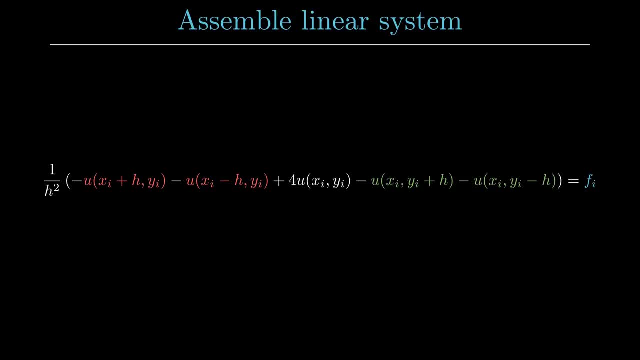 squared times minus u of xi plus h comma yi, minus u of xi, minus h comma yi, plus four times chi plus h comma yi, minus one over h squared times pi over h squared u of xi yi minus u of xi yi, plus h minus u of xi yi minus h, which equals fi. 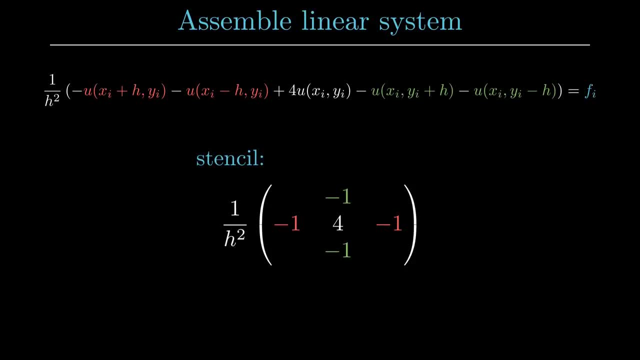 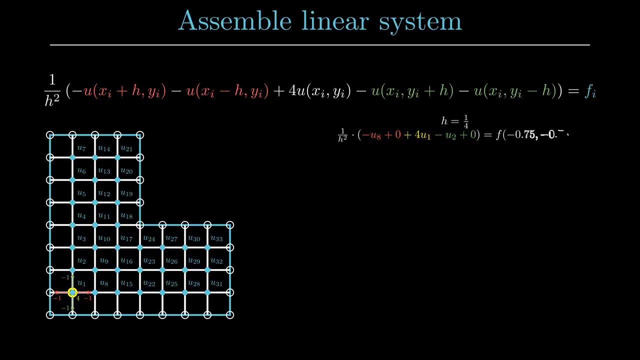 This difference quotient is known as the five-point stencil and can be represented by this matrix. Going back to the decomposed domain, we now go over all grid points and show the equations that we get from applying the stencil. When applying the stencil, we also account for the fact that the function u equals zero. 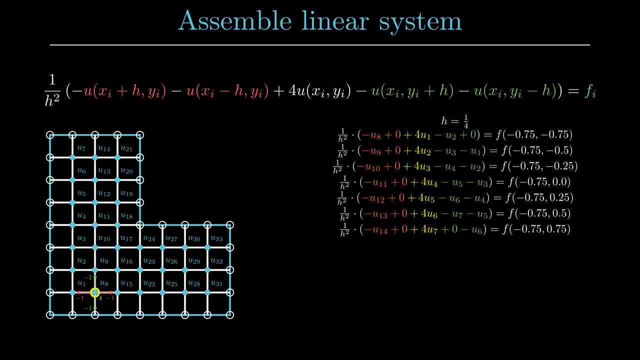 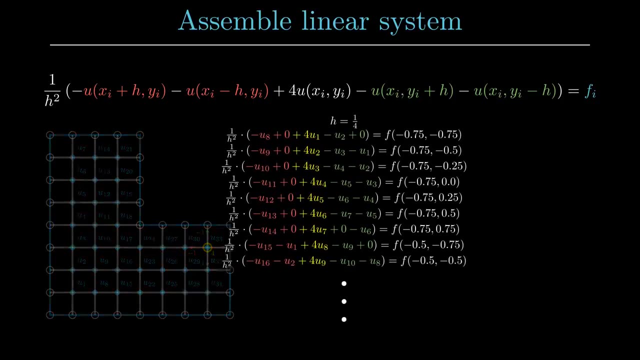 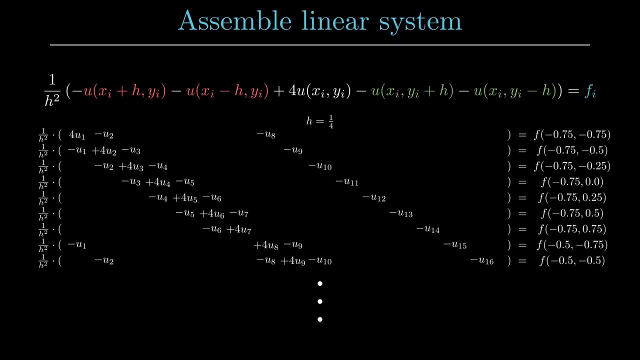 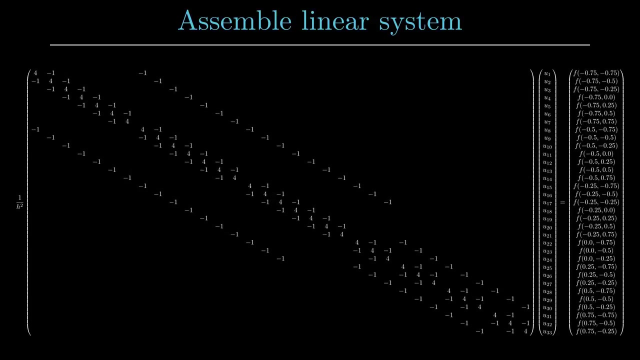 at the boundary. After looping over all grid points, We can now regroup the equations, which can also be written down in matrix notation. Overall, we get a linear equation system with 33 unknowns which can now be solved if the right hand side function f is given.